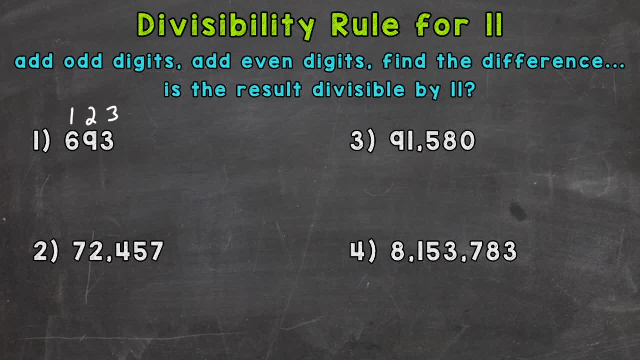 And 9 is the even digits. So let's add our odd digits 6 and 3, I'll put odd equals: 6 plus 3 is 9.. And even. Well, we just have one digit and it's a 9.. 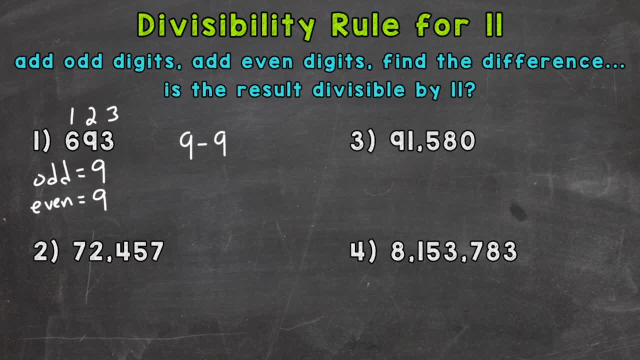 So let's find the difference. So 9 minus 9 equals 0.. So this is our difference, and we need to see if that is divisible by 11.. 0 is divisible by any number. therefore it's divisible by 11.. 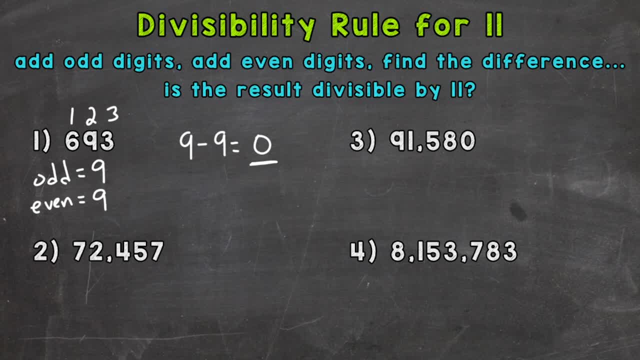 Since our result is divisible by 11,, that means, our original number 693, is divisible by 11 as well. Let's try this again with number 2.. So we have 72,457.. So let's count our digits. 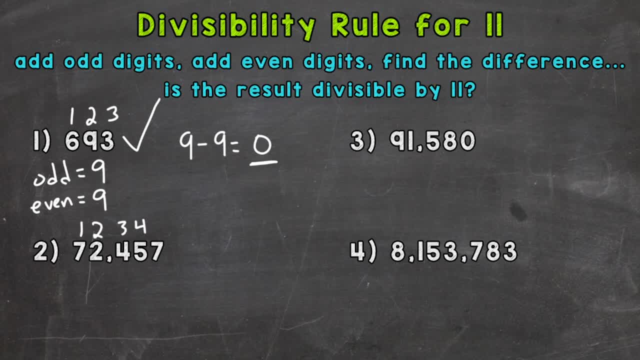 1,, 2,, 3,, 4, and 5.. So odd, and even So, the odd digits: 7 plus 4 is 11.. So 7 plus 4 is 11, plus 7 is 18.. 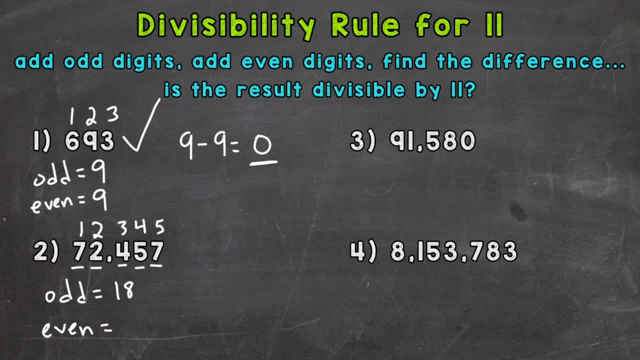 The even digits. Well, we have: 2 plus 5 is 7.. So let's find the difference here. We have 18 minus 7, which gives us 11.. 11 is divisible by 11,. therefore our original number, 72,457, is divisible by 11.. 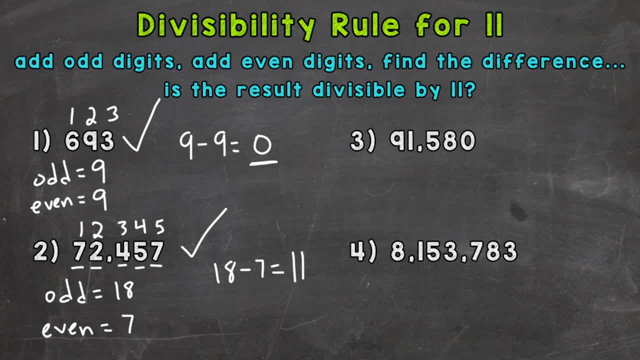 On to number 3, where we have 91,580.. So let's count off 1,, 2,, 3,, 4.. 5.. So odd and even So odd, we have: 9 plus 5 is 14, plus 0. 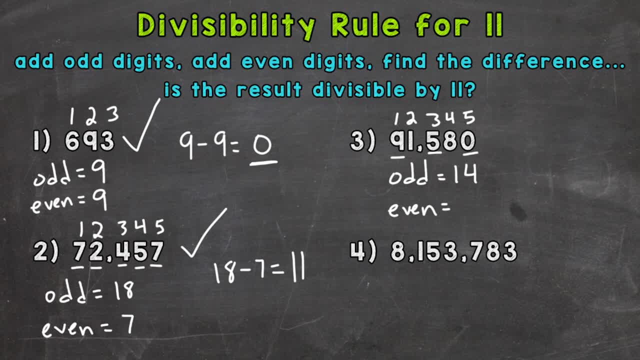 So we end up with 14 here. Now, even we have 1 plus 8,, which is 9.. So 14 minus 9 gives us 5.. 5 is not divisible by 11,, therefore 91,000..